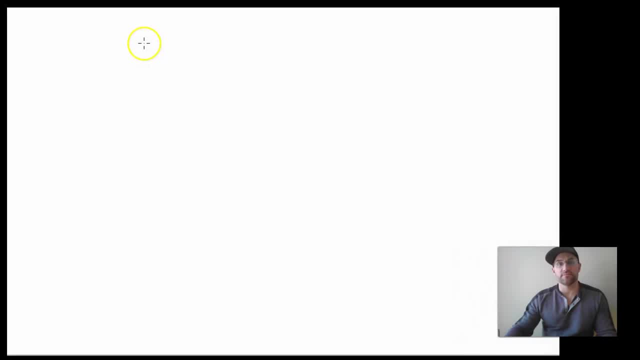 Alright, guys, we're going to do another complex number. This time we're going to have some fractions or rational numbers, right? When we see the word rational numbers, what we should see is ratio, right, Because a fraction is a ratio, a fraction is a decimal, is a percent, is a rate of change, is a slope, it's a division problem. 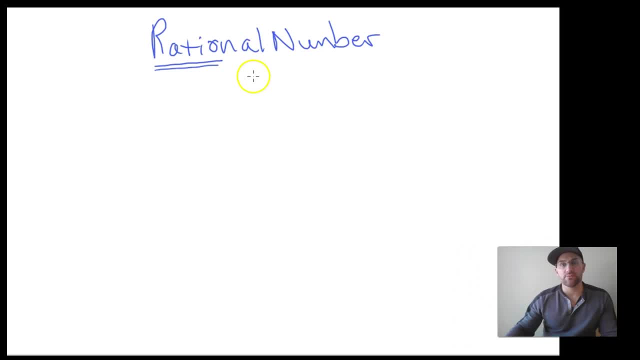 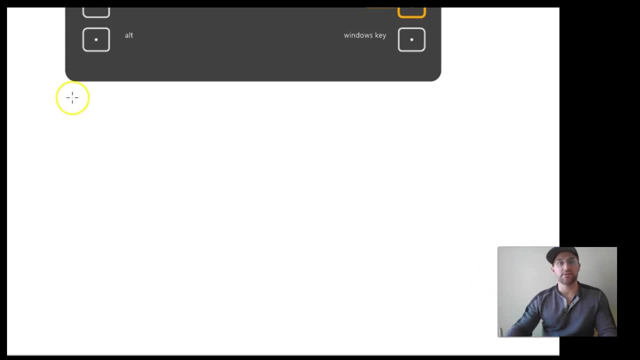 They're all the same thing, right? So a rational number is a fraction. We see the word ratio right there. okay, So let's not get intimidated by those. And we're going to see some fractions in the form of, or we're going to see some complex numbers with fractions. 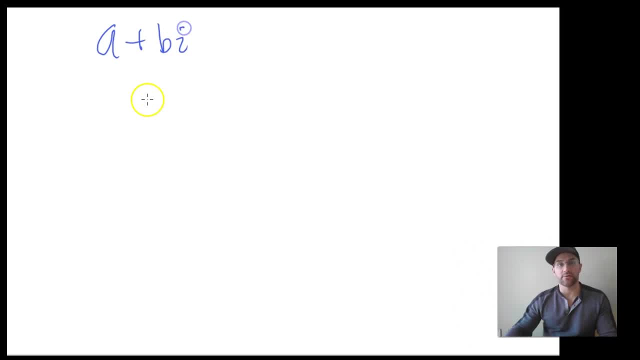 So remember the form A plus BI, right? So this is the real part, this is the imaginary part. Well, let's go ahead and look at the problem We have. I have it written down here. I wrote some down here, right here. 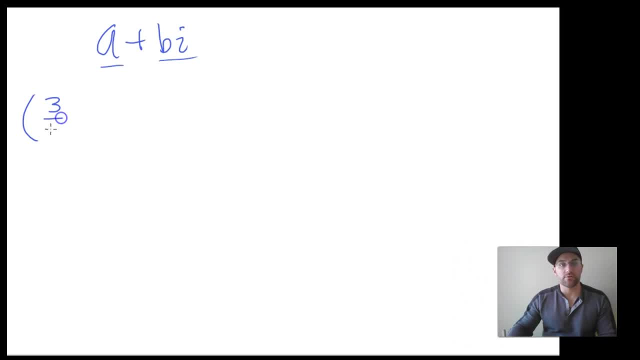 Alright, so we're going to have three halves, or three over two. that's positive. positive five-eighths I, right. So A positive BI, right, It's nothing to be intimidated by. So when we add that to negative one-fourth, positive one-fourth I, this is also right. 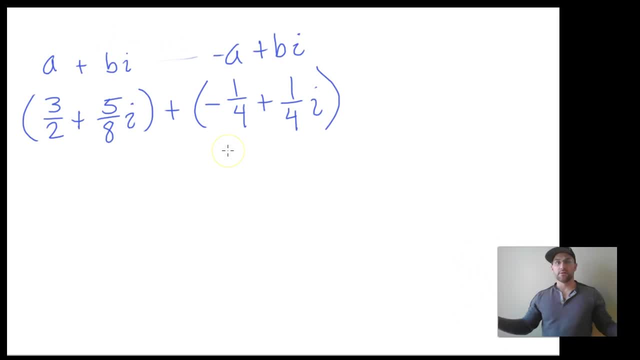 Plus BI. now it's negative, A right, No problem. And we remember. when we add complex numbers, all we do is we take the real part- and here's our real part, right, We add it to the other real part. 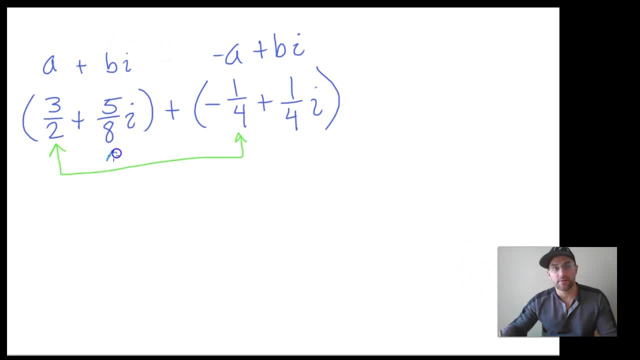 We take our imaginary part right here and we add it to the other imaginary part, right? So what do we have? We have three halves plus minus one-fourth. So we have three halves Plus minus one-fourth, right. 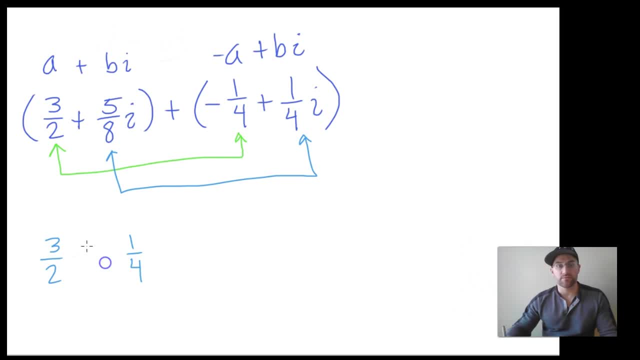 So we can just get rid of that plus and just make it minus one-fourth, right. So we have three halves. take away one-fourth. We need to find the lowest common denominator, right, And we can see that that's going to be four. 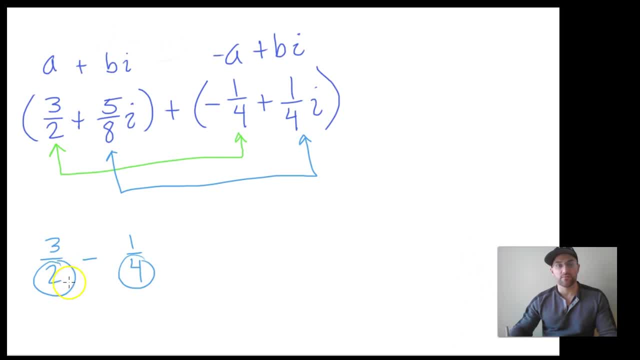 So how do we increase this three halves to a fourth in the denominator position? Well, we multiply by two. Whatever we do to the bottom the denominator, we have to do to the top, which is the numerator right, Because it's a ratio.